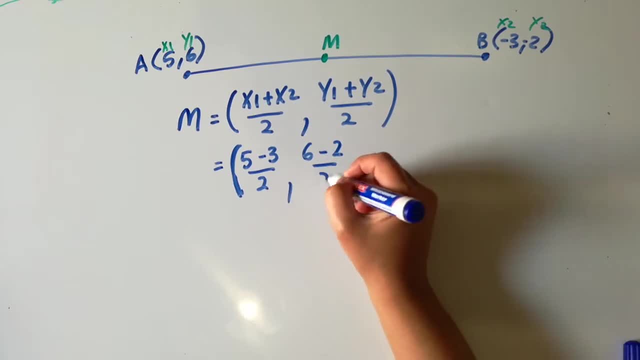 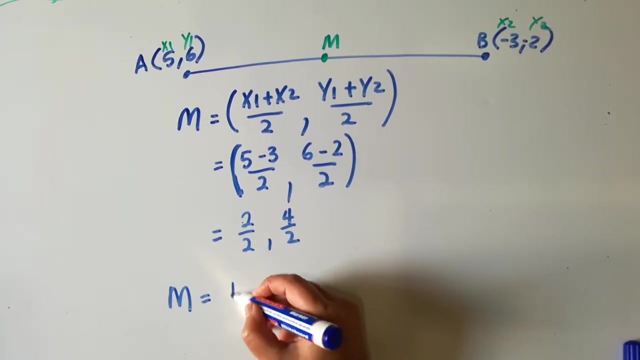 say plus minus 2, I'm going to get minus 2 divided by 2. 5 minus 3 is 2 and 6 minus 2 is 4. so the coordinates of M will have an x coordinate of 2 divided by 2 is 1. 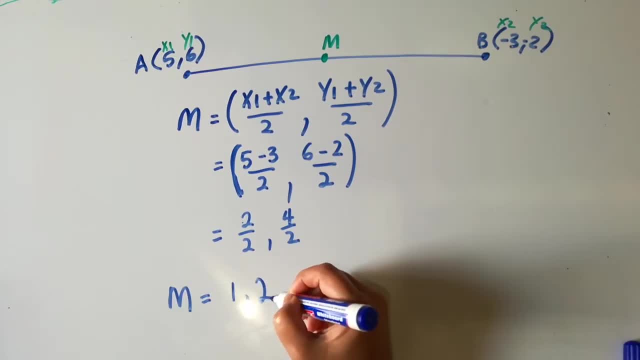 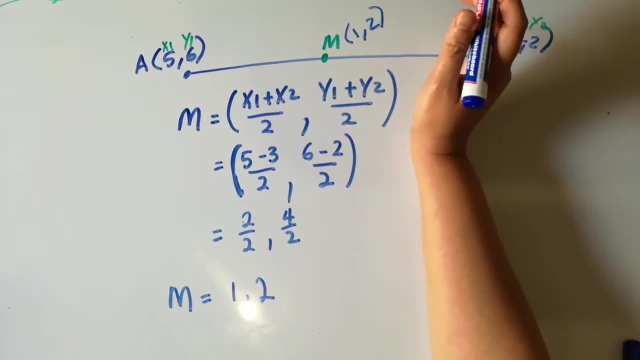 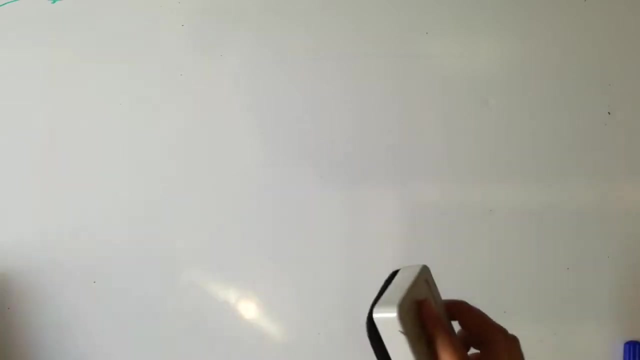 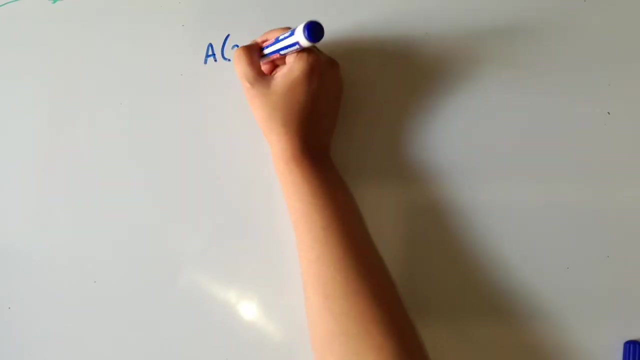 and 4 divided by 2 is 2. so here we have x1 and y is 2, easy. let's do something a little bit different, harder. let's say I have two points: point a, which has an x coordinate of 2, y coordinate of 7. b, where we don't know what the x coordinate is. we don't know. 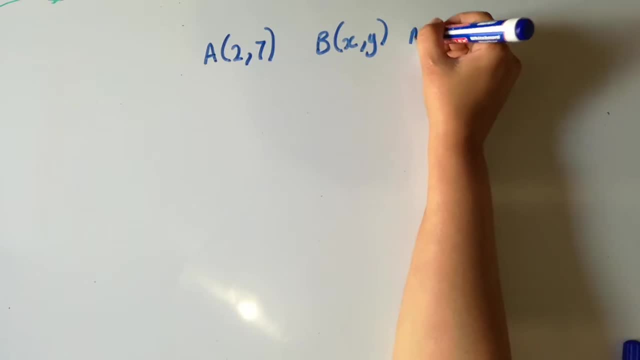 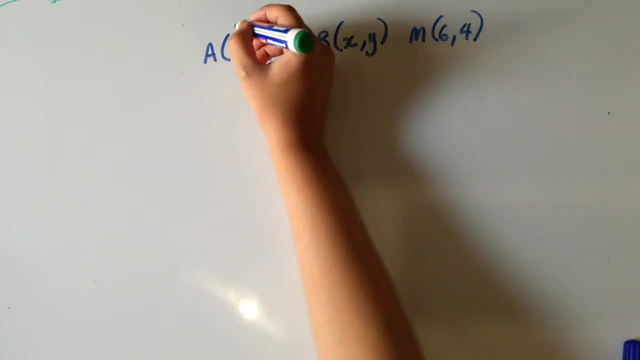 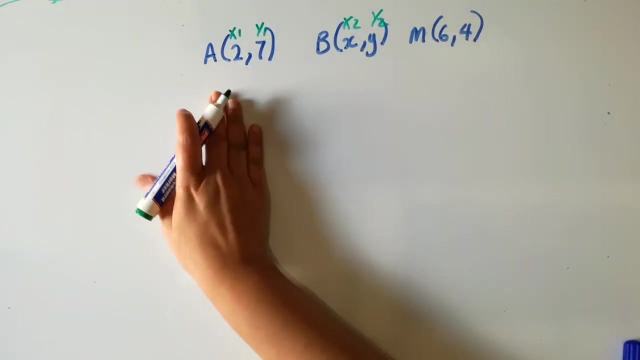 what the y coordinate is, but we do have the coordinates for the midpoint, which is 6 and 4, so let's label this before we begin. that's x1, y1, y1, x2 and y2. I like to calculate the x coordinate separately and the y. 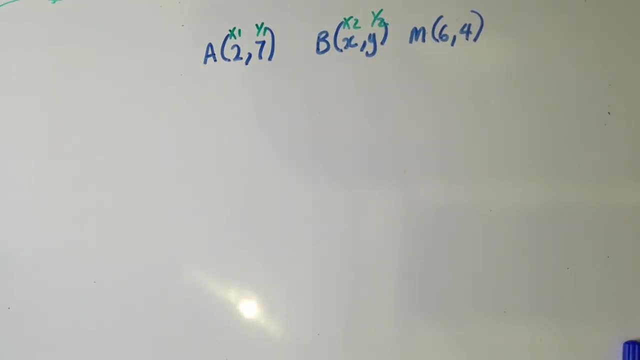 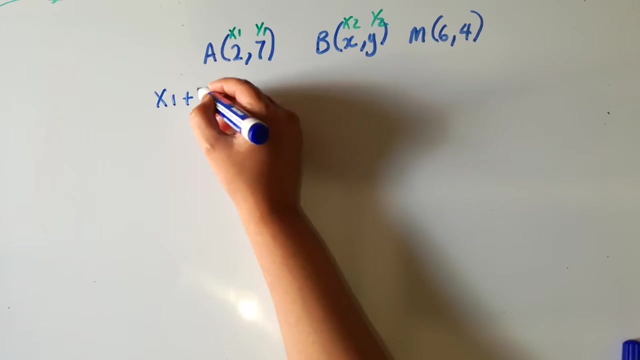 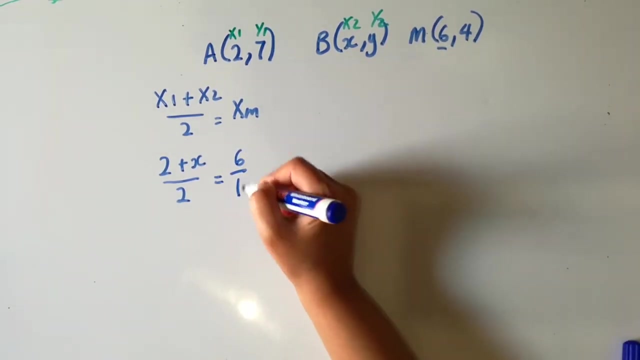 coordinate separately. I find that to be less confusing. so we know. to find the midpoint x, I'll say x1. his 2 divided by two will give me the midpoint X, so that x1 is 2, x, 2 is x, x2 is x. divided by 2 will give me this x value here, 6 over 1. why did I write it as a? 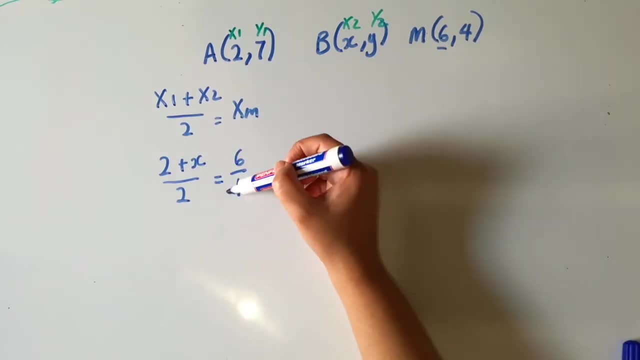 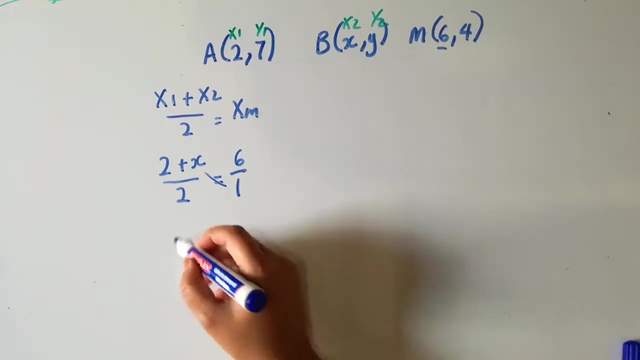 fraction, because to solve for X here I'm gonna have to cross multiply, and if I cross multiply I'm gonna need it to be a fraction. so 6 as a fraction is 6 over 1. if I cross multiply, 2 plus X times 1 will give me 2 plus X and 6 times 2 will. 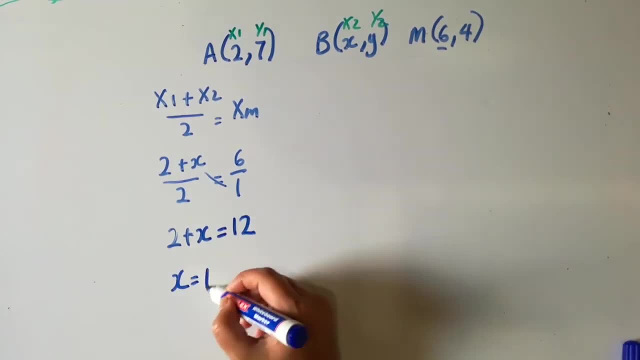 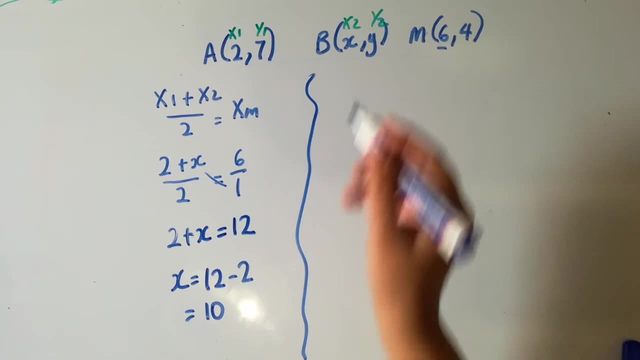 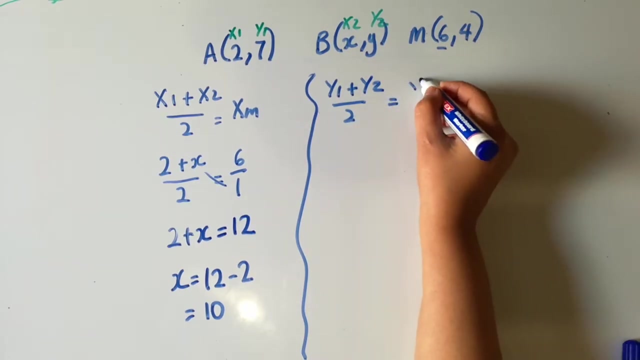 give me 12. therefore, X is equal to 12 minus 2, which will give me 10. I'm going to do the same thing for the y coordinate. I'm gonna say Y 1 plus Y 2, divided by 2, will give me the y coordinate of the mud point.